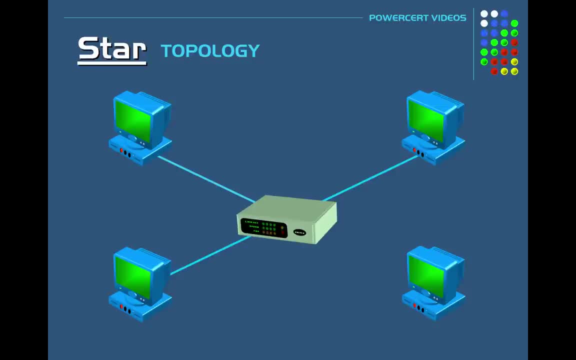 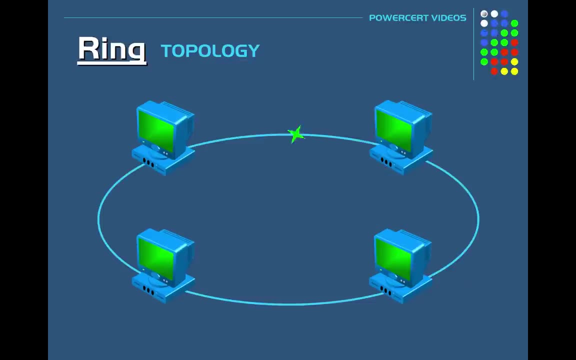 a single point of failure. If this happens, the entire network goes down. Another type of topology is called ring. The ring topology is a type of network configuration where each computer is connected to each other in the shape of a closed loop or ring, So every 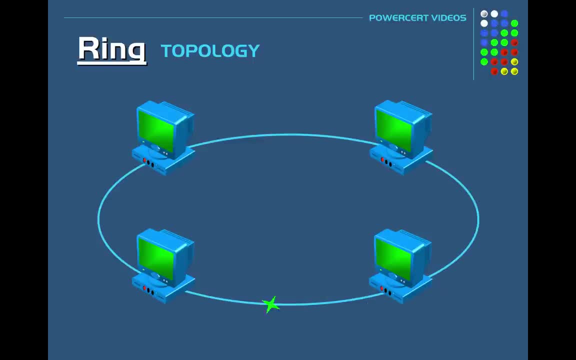 computer on this ring has exactly two neighbors. for communication purposes, Each data packet is sent around the ring until it reaches its final destination. Now, this kind of topology is very old and is rarely used today. Now, the advantage of a ring topology is that they are easy to install and 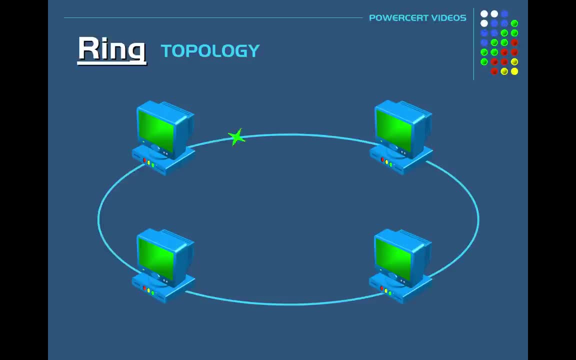 easy to troubleshoot. Now, the advantage of a ring topology is that they are easy to install and easy to troubleshoot. However, the disadvantage would be that if just one of these computers goes down, or if there was a single break in the cable, then all data flow would be disrupted. 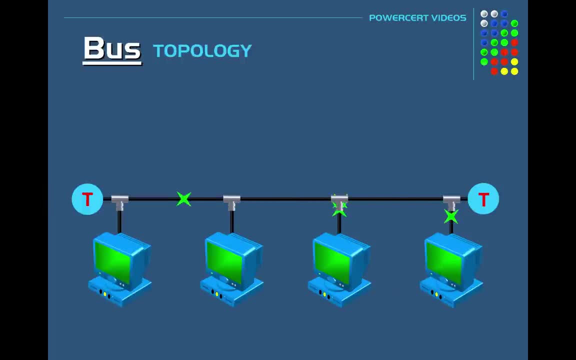 And the next one is the bus topology. The bus topology is very old technology and, like the ring topology, it's not used today that much. This is the kind of network setup where each of the computers in parallel and in parallel have the same 12-tab technology as the main one. 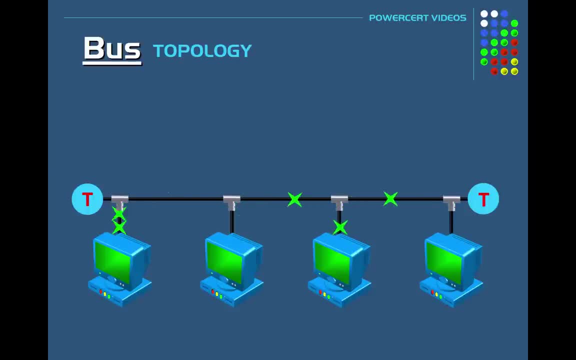 This is the type of network setup where you can now connect. network devices are connected to a single cable or backbone, and this backbone is a coaxial cable. The computers connect to this cable using special connectors called BNC, which are also known as T-connectors. One of the advantages of the bus topology is that it is also fairly cheap and 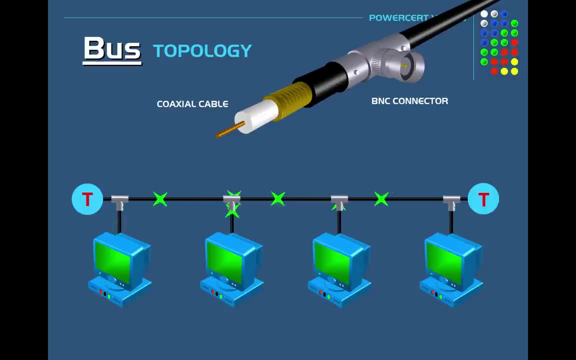 easy to implement. However, a disadvantage of the bus topology is that it requires that the cable be terminated at both ends using terminators. In order for this setup to remain operational, there must not be any open connections, including the ends that attach to the computers. So if a computer 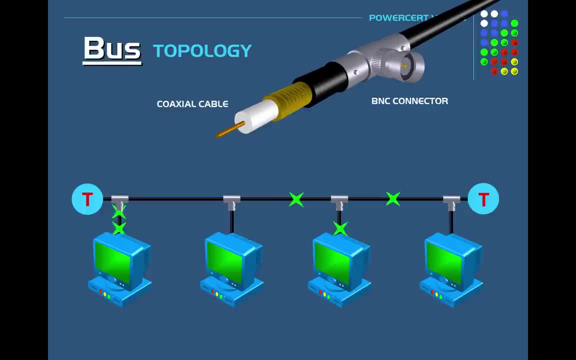 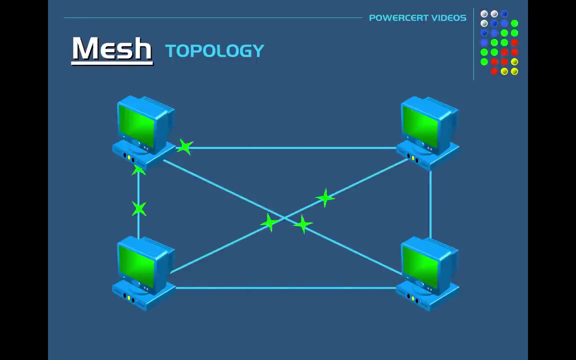 is removed, or if the terminators are loose or missing, then the cable would be open and then data would bounce back, and this bounce is known as signal reflection. and if this happens, data flow would be disrupted. And there is also the mesh topology. Now, in a mesh topology, each computer on the network is connected. 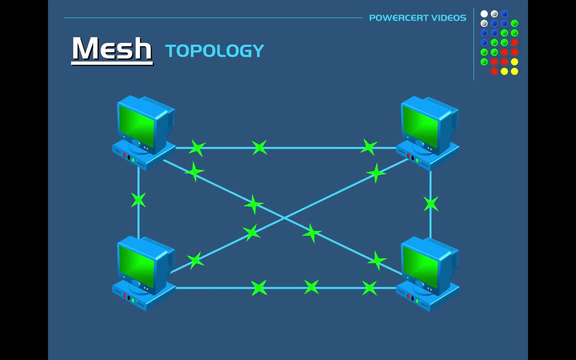 to every other computer on the network. so by having so many connections it handles failure very well. In this illustration there are four computers with three connections on each computer, which makes a total of 12 connections for this network. Now, the advantage of a mesh topology is: 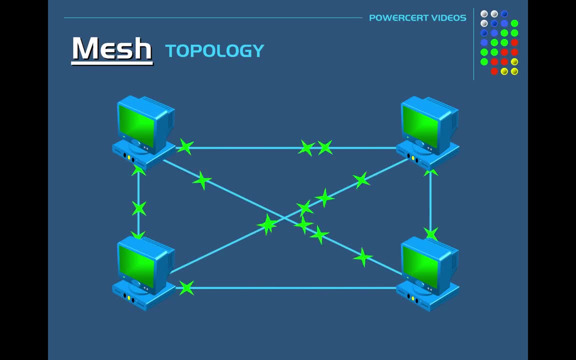 that it creates a high redundancy level, because if one or more connections fail, the computers would still be able to communicate with each other. However, because of the amount of cabling and network cards that have to be used, mesh topologies can be expensive, so they are rarely used on local area networks or LANs. 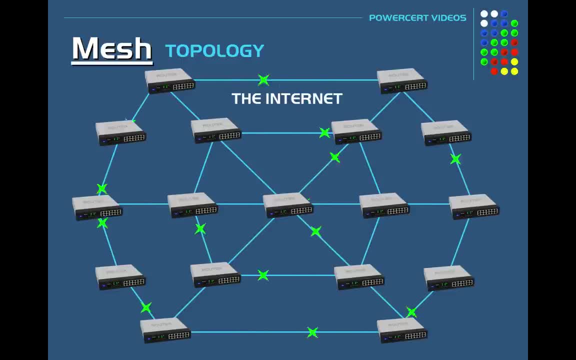 They are mainly used on wide area networks like the internet. In fact, the internet is a good example of a mesh topology, because the internet is made up of numerous routers all over the world that are connected to each other to route data to their intended destination. So even if a few 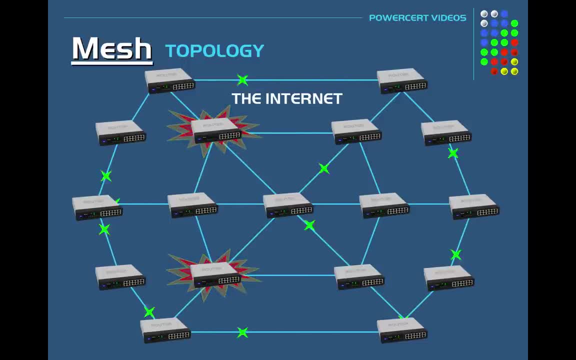 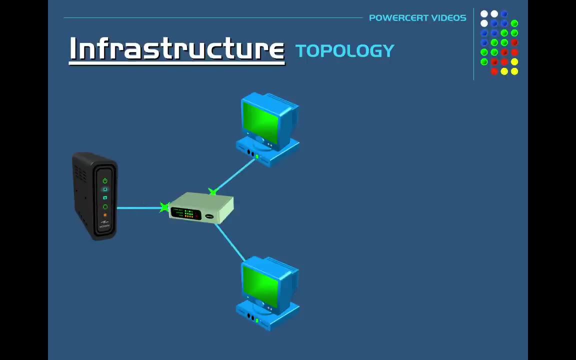 routers go down, the data will get rerouted, using a different path to ultimately reach their destination. So the internet is very redundant because it's using a mesh topology. So now we're going to talk about wireless topology. So let's start with the infrastructure: wireless topology Now. this topology uses a combination of: 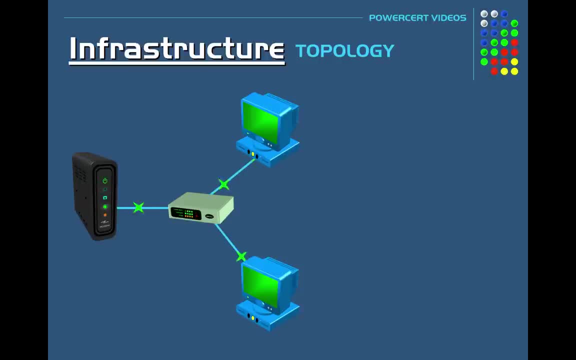 wired and wireless devices. Now, this is very similar to a star topology, where you have wired devices, such as these computers here, physically connected to a switch and you also have a wireless access point that's also connected by a cable to the same switch. The wireless access point is here. 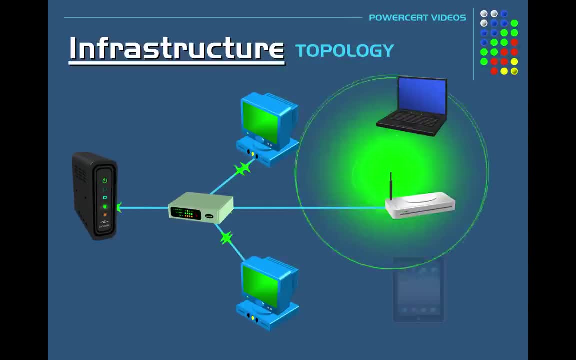 so that wireless devices such as laptops, tablets, cell phones etc. can connect wirelessly to the network. So the wireless access point acts like a bridge between the wireless network and the wired network. Now the infrastructure topology is not limited to a single wireless access point. In fact, 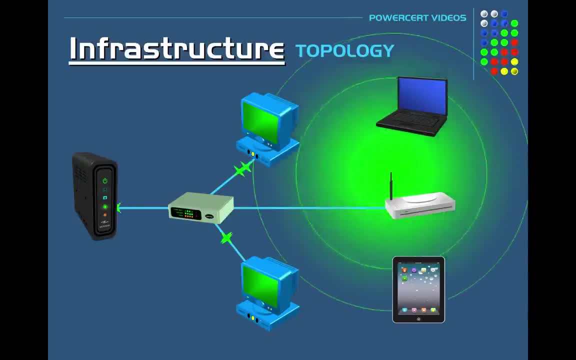 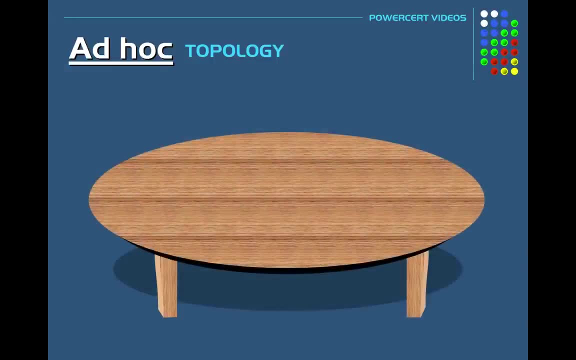 you can have multiple wireless access points if you want. It just depends on the needs of the network. And the next wireless topology is ad-hoc. Ad-hoc is a very simple wireless topology and it's simple because it doesn't rely on any infrastructure such as cables, routers, servers. 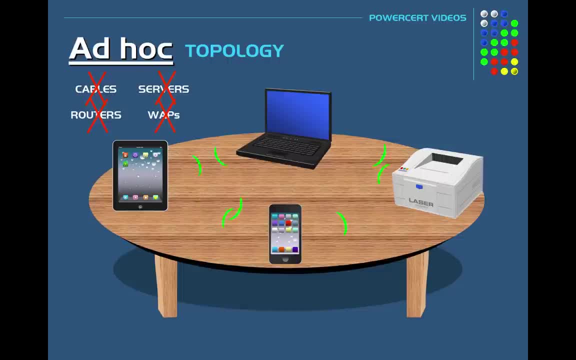 or wireless access points. All the devices in an ad-hoc network wirelessly connect to other devices in a simple peer-to-peer network. They directly connect to each other without using a centralized network. So if you have an ad-hoc network and you want to connect to a wireless network, you can. 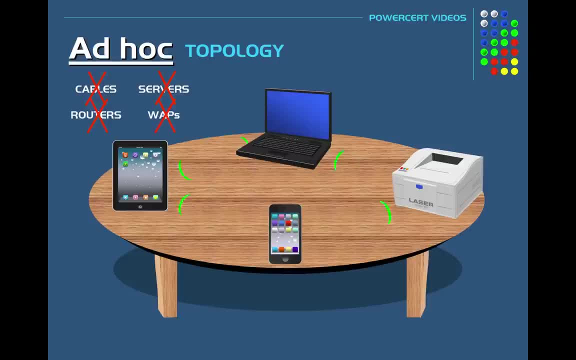 use a centralized device such as a Wi-Fi router or access point, And because they directly access each other without a server or router in between, each device is responsible for its own security and permissions. Ad-hocs are useful for setting up a quick wireless network on the fly where devices 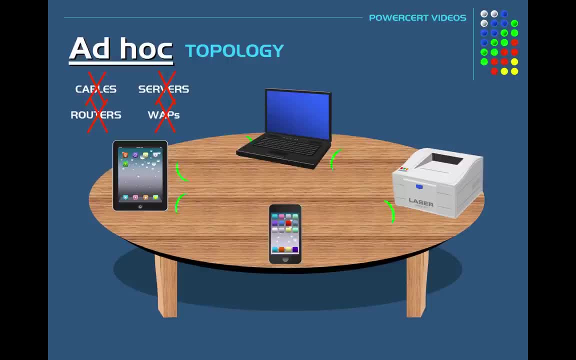 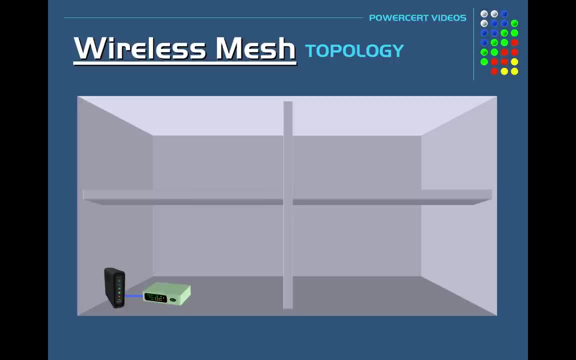 can share data without the need of an existing wireless network, And the last wireless topology is called a wireless network And the last wireless topology is called a wireless network And the last wireless network is called a wireless mesh. Wireless mesh topologies are similar to wired. 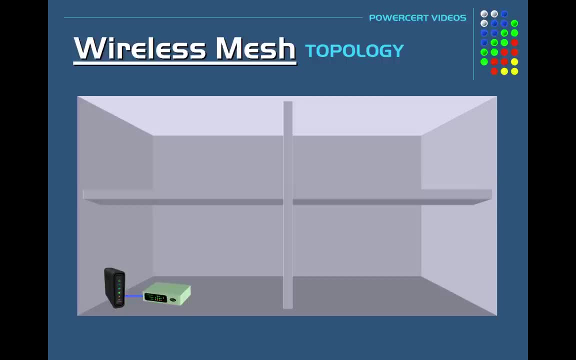 mesh topologies, where devices are interconnected with each other, but with the exception that they are wirelessly interconnected. So, for example, let's say you wanted to deploy multiple wireless access points all throughout a building so that wireless devices that are in different areas 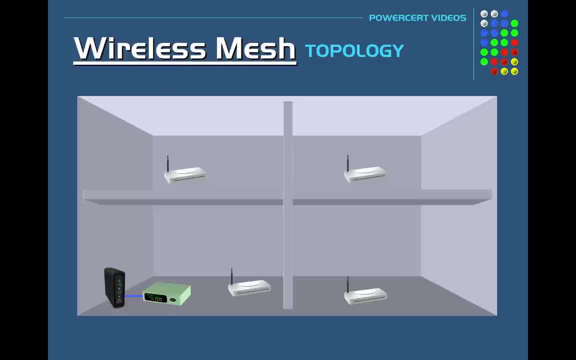 are able to access the internet. So normally you would have a modem that brings in the internet to the building, And then you would also have a switch that's connected to the modem, And then you would connect each wireless access point with a cable to the switch. So by doing, 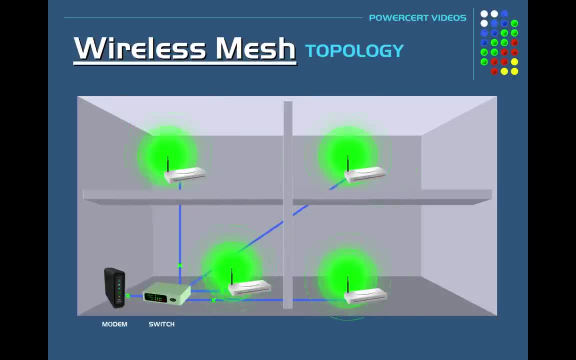 it this way. this requires extra cabling and it would also require extra time running the cables through the building. So this is more expensive and more time consuming. Now a wireless mesh topology would be similar to this setup, But the need of these extra cables. In a wireless mesh each wireless access point will talk to. 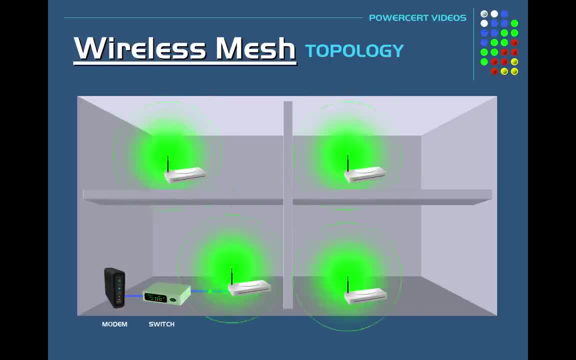 other wireless access points to create a seamless internet connection for wireless devices to connect to. So if this laptop over here wanted to access the internet, it would connect to the nearest wireless access point and then this access point would relay the connection to the next access point and then to the next one and then eventually find its way back to the modem. So no,